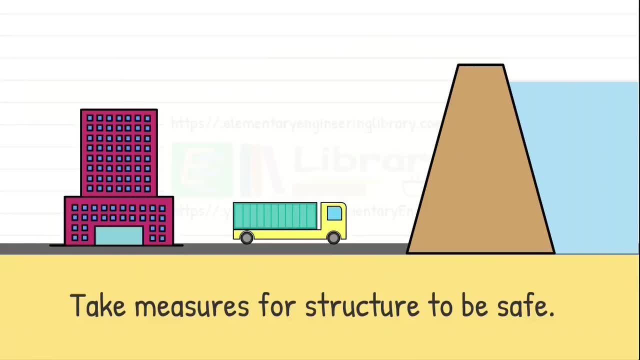 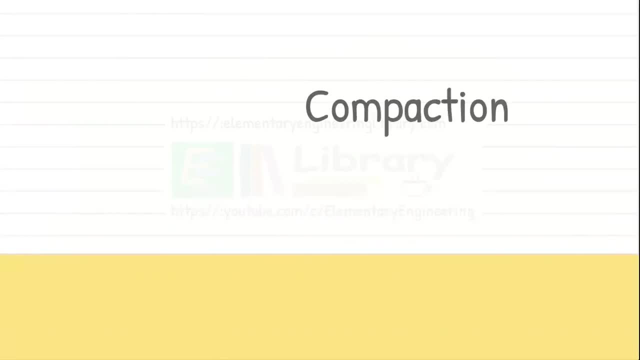 and don't get damaged by undesired settlement. The process of making soil base solid before the construction is called compaction. Compaction is the process of application of mechanical energy to the soil. Because of this, soil grains get rearranged more closely, the volume of air voids get reduced. 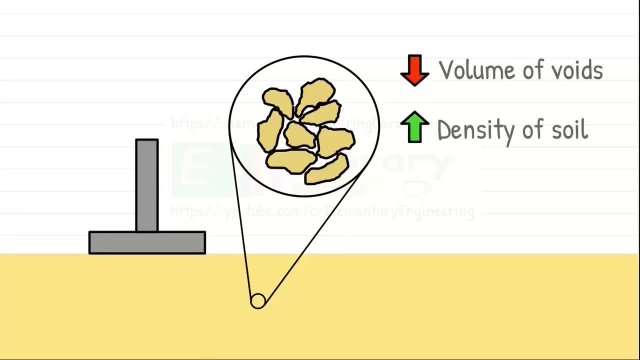 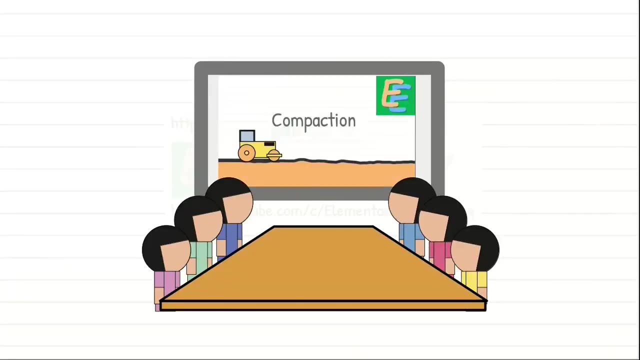 and the density of soil increased. Higher the density of soil, stronger the soil is. By strong we mean it has higher shear strength and bearing capacity. We have discussed all these in a little more detail in our previous video. You can find the link to that video in the description or in the i button above. 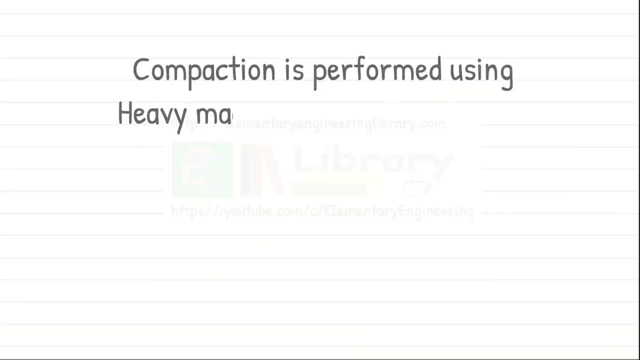 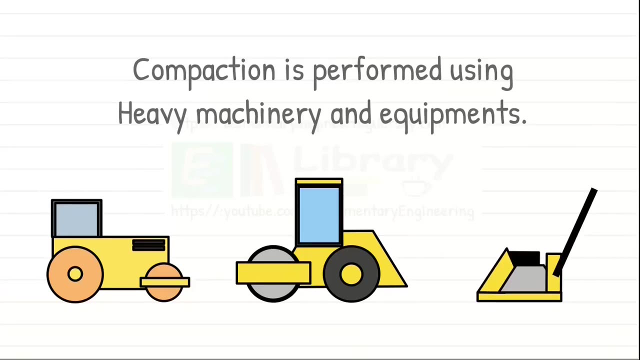 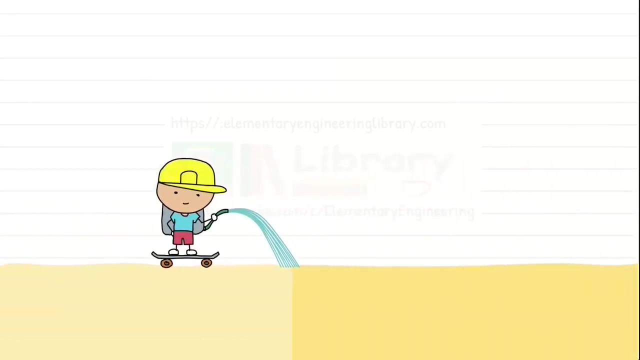 Compaction is usually done with heavy machinery and equipment such as vibratory compactors, rollers or compacting plates. By doing compaction for many years now, we found that if we add a little water to the soil and then try compacting it, it gets better compact. 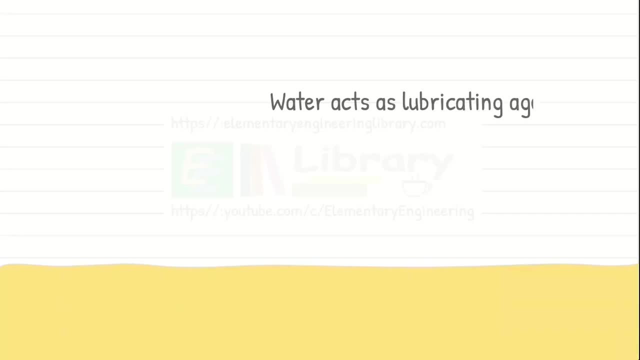 Because water acts as a lubricating agent between the soil particles. When the load is applied to the soil, the water between the soil particles helps them move more easily and helps soil achieve denser configuration. but how much water we need for a good compaction, and what is a good compaction? how do we know we have done? 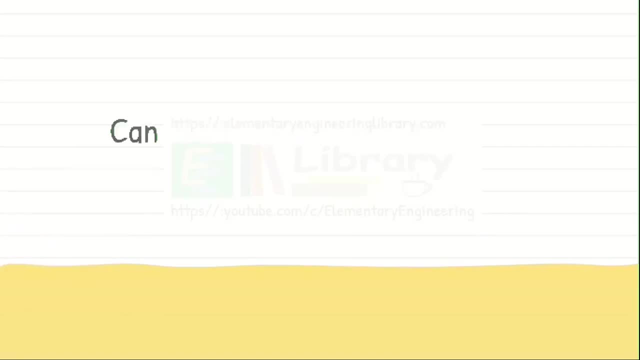 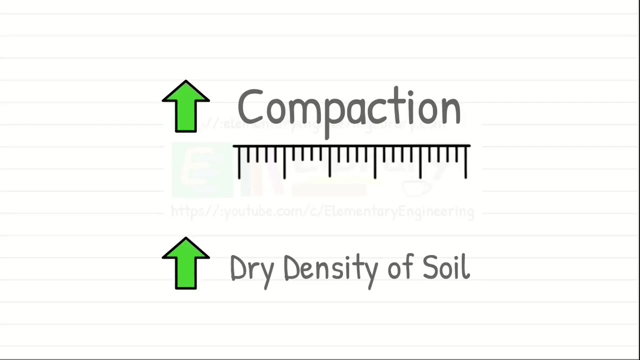 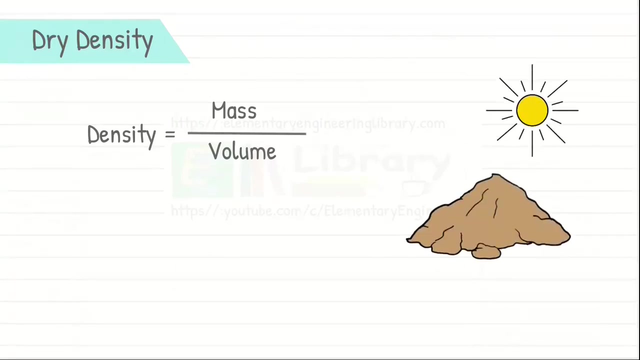 enough or we need more of it. is there any way we can quantify the compaction? well, yes, the amount of compaction is measured by the dry density of soil. higher the dry density, higher is the compaction. dry density is the density of soil when soil is in completely dry state, which means no water is present in. 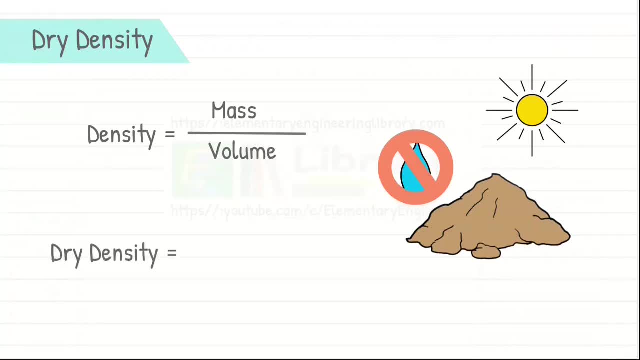 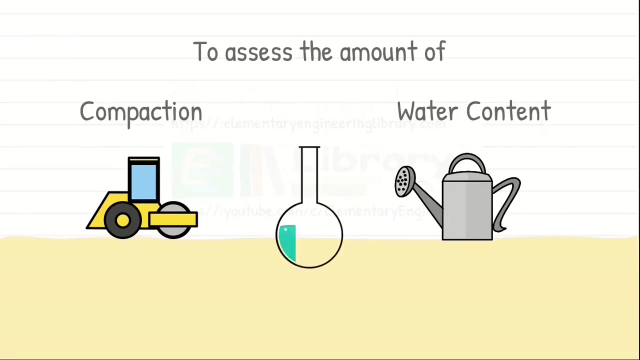 its pores. so the dry density of soil is mass of soil solids only divided by its volume. to assess the amount of compaction and the water content required in the field, we perform a laboratory tests on soil. these tests provide a relationship between the water content and the dry density of soil. typically, the procedure 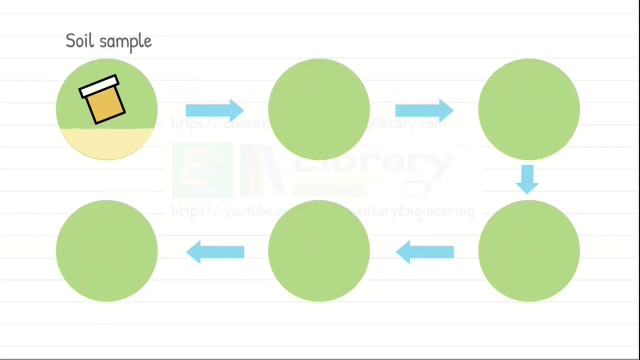 is that that we collect a soil sample from the site and perform laboratory tests on it. we obtain results that are satisfactory to us for the level of compaction we require. then we perform compaction in the field and during the process, perform tests in the field to verify that compaction in the field is. 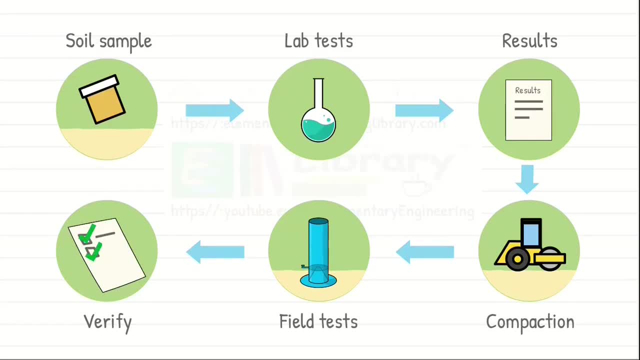 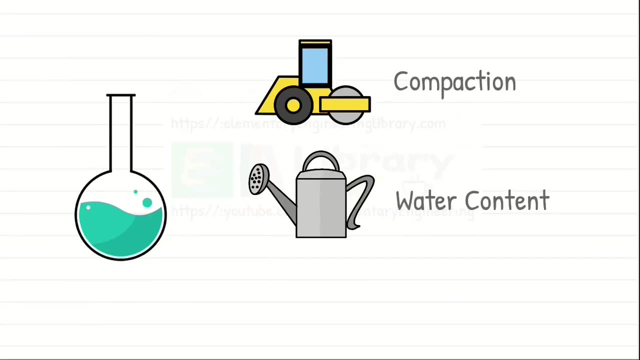 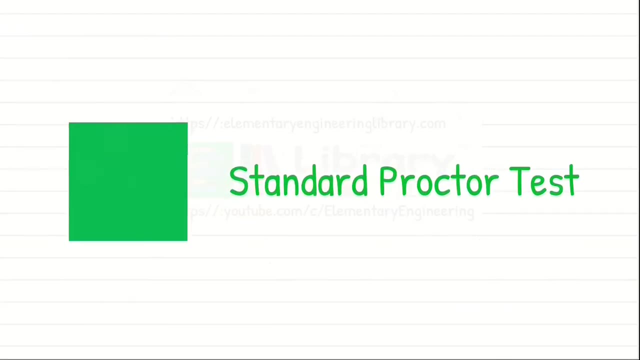 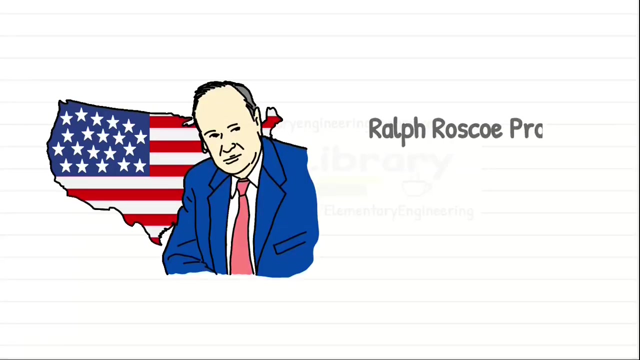 consistent with the lab results. One such laboratory test that is used to determine the amount of compaction and water needed for different types of soil is standard proctor test. American civil engineer and soil scientist, Ralph Roscoe Proctor, developed the principles of soil compaction He found through his 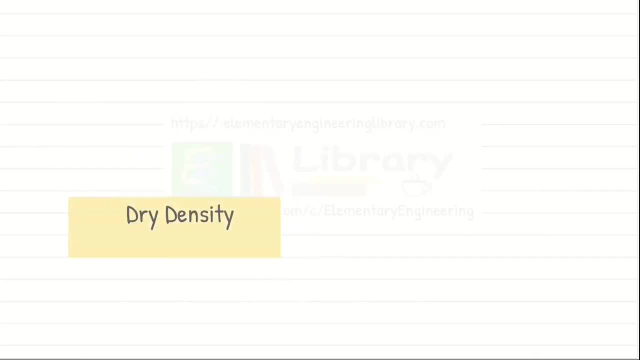 experiments that the dry density of a soil for a given compactive efforts depends on the amount of water the soil contains during soil compaction. In simpler words, he found a relationship between the difference between soil density and the amount of water the soil contains during soil compaction. In simpler words, he found a relationship between the 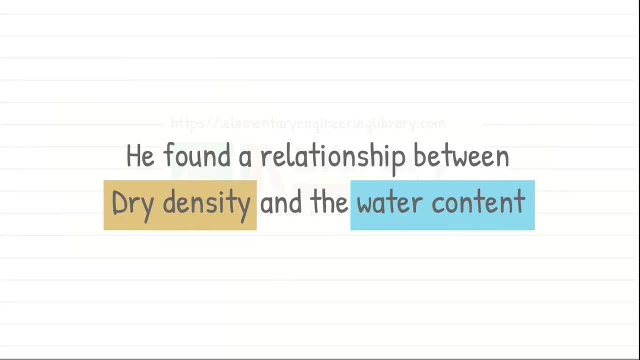 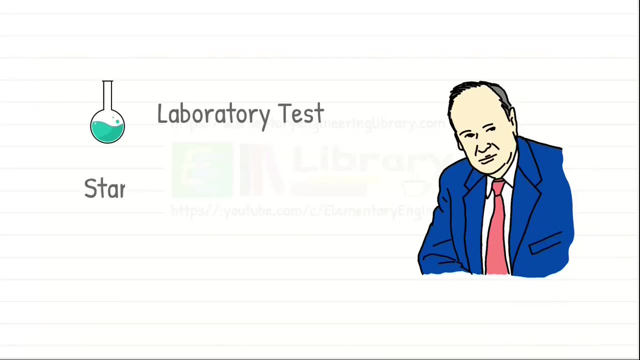 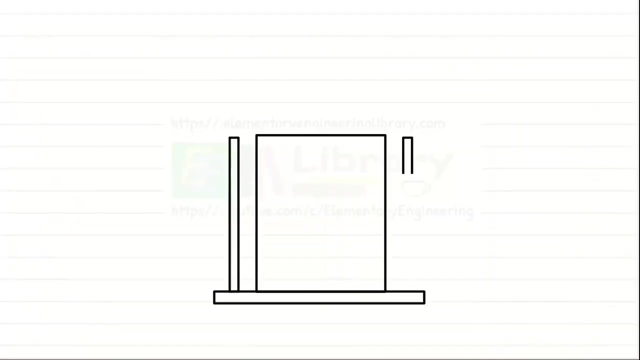 dry density and the water content of soil As a tribute to Proctor. the laboratory test that he devised is called standard proctor test or proctor compaction test. In this test, specified amount of compactive effort is applied to a constant volume of soil mass. For the test we use a standard mold of internal diameter of 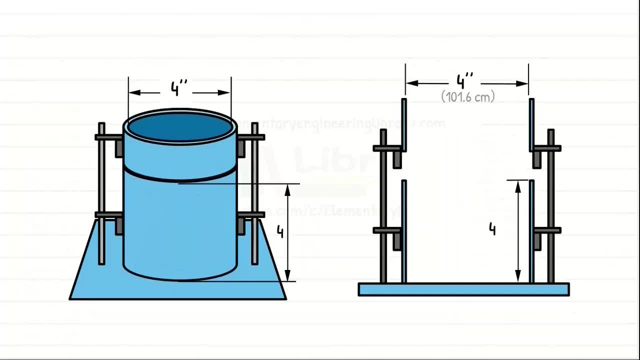 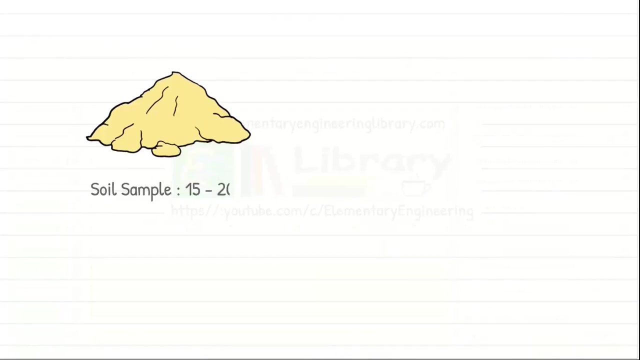 4 inches and an effective height of 4.5 feet inches. Its standard volume is 1 by 30 cubic foot. It also has a detachable base plate and a removable collar of 2 inches height at its top. We collect a soil sample of about 15 to 20 kg from the 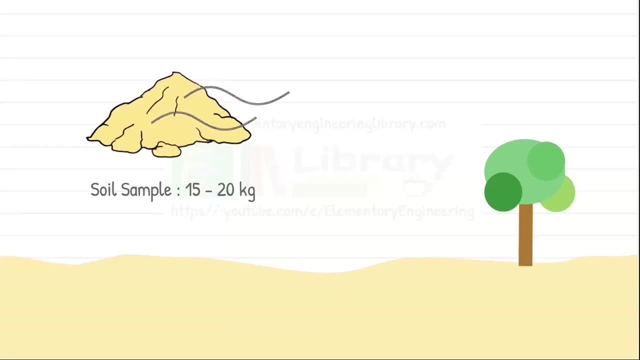 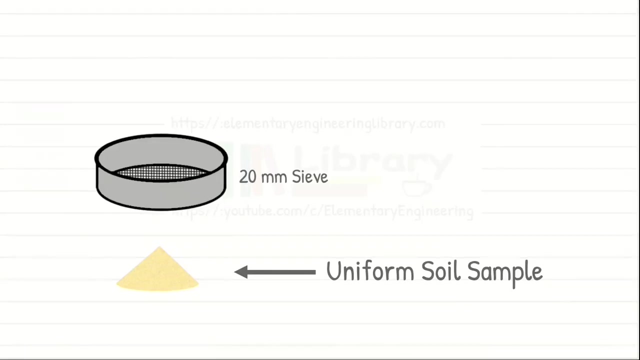 field. We air dry the soil and remove it. We remove any organic material or debris present in it. Then about 5 kg of sample is crushed and passed through 20 mm sieve so that we can have a uniformity in our soil sample. The soil passing through the sieve is taken. We add a little water to. 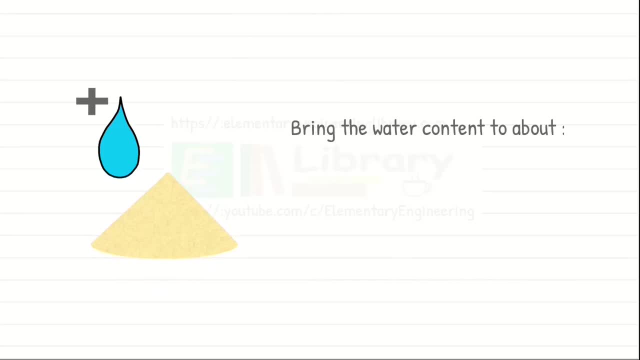 the soil so as to bring its water content to about 4% if the soil is coarse grit and 8% if it is fine grit. but how do we know how much water is needed to bring the required percentage of water content? Well, water content is a weight of water divided by a weight of solids present in the soil. 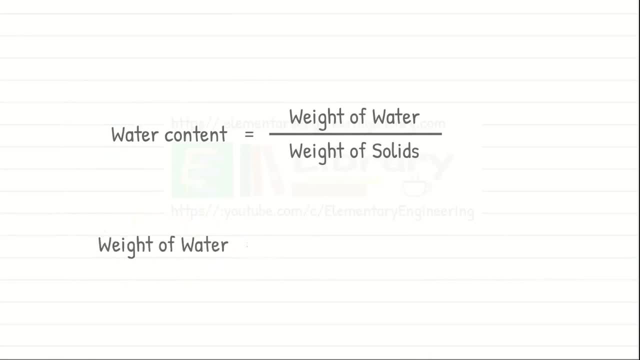 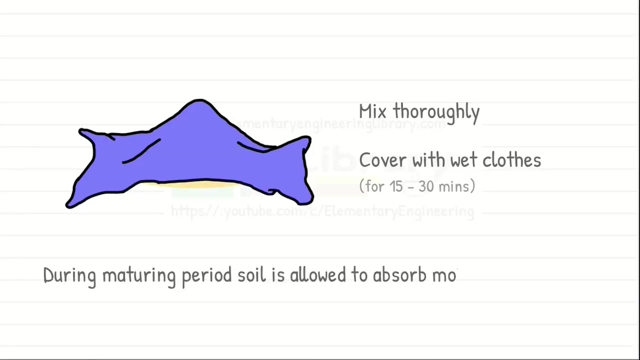 So weight of water can be calculated as a water content multiplied by weight of solids. Now the soil is mixed thoroughly and covered with a wet cloth and left for maturing for about 15 to 30 minutes. During this period, the maturing period, soil is allowed to absorb moisture uniformly. after mixing The 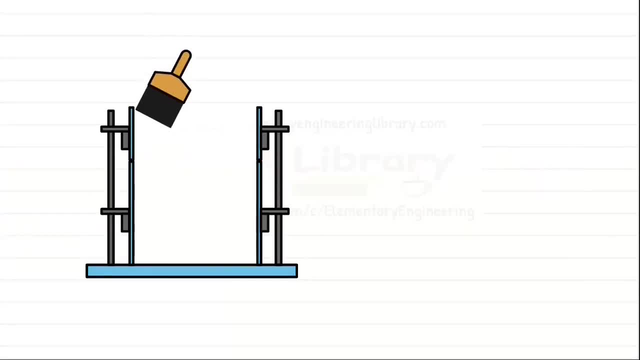 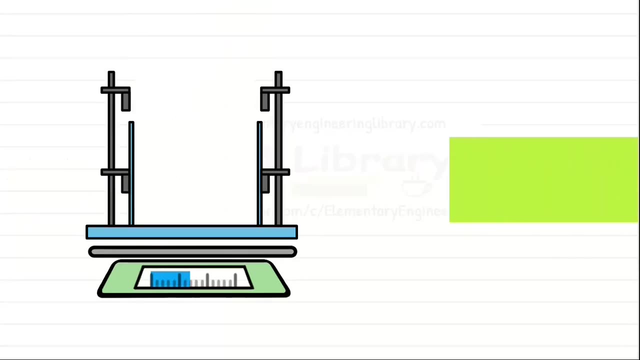 mold is cleaned, dried and greased lightly so that soil does not stuck with the mold. The weight of empty mold with the base plate but without collar is taken and noted down as W1.. The collar is then fitted to the mold and it is. filled with the soil to about one-third its height. Soil is compacted by a rammer of weight: 5.5 pounds, approximately 2.5 kg. It is allowed to fall freely from a height of 12 inches. 25 number of such blows are. 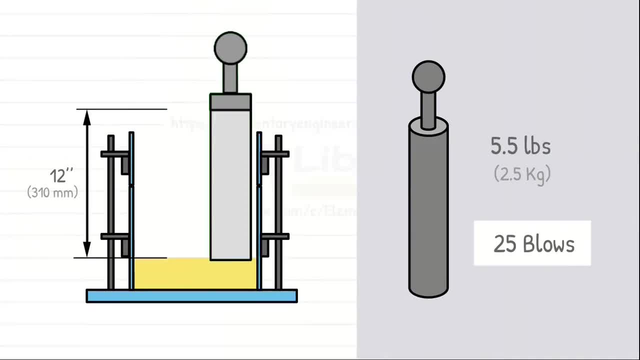 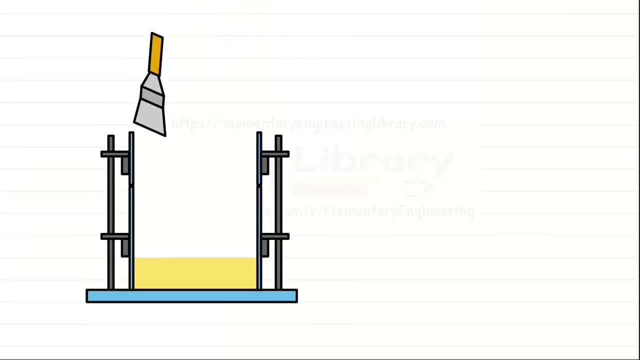 given and they should be evenly distributed over the surface of soil. Then, before adding the second layer of soil, we scratch its surface with a spatula. We fill the mold with soil to about two-thirds of its height and compact it in similar way by 25 blows of rammer. Again, soil is scratched. and third layer: 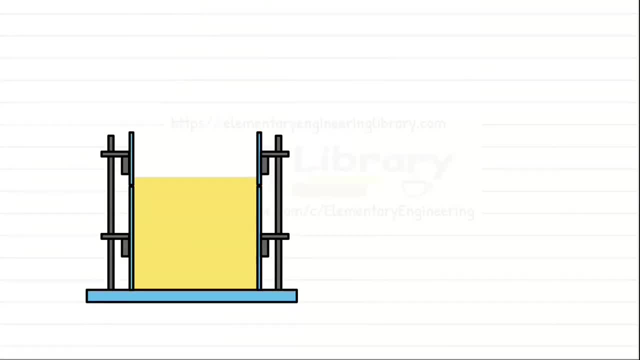 of soil is placed into the mold. The final layer should project a little above the top of the mold in the collar, but not more than 6 mm. The layer is compacted in the same way. Then we remove the collar and trim the excess soil off The mold with the base. 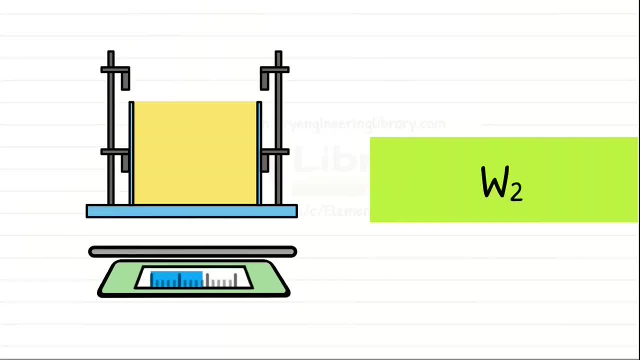 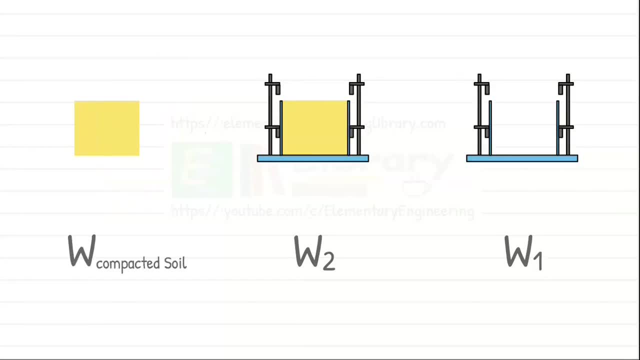 plate is weighed and noted down as W2.. Hence we can determine the weight of compacted soil as W2-W1. At this stage we know the volume of mold and weight of compacted soil, So we can calculate the bulk unit weight of this compacted soil, where W is the weight of. 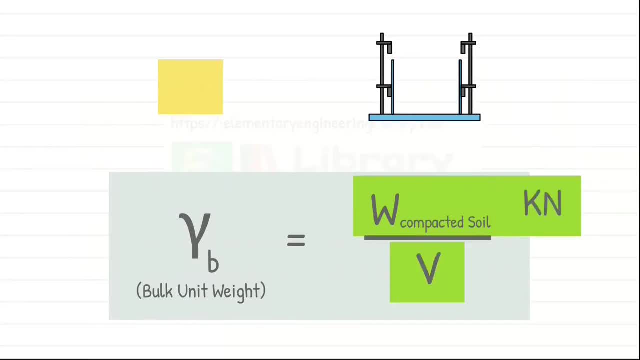 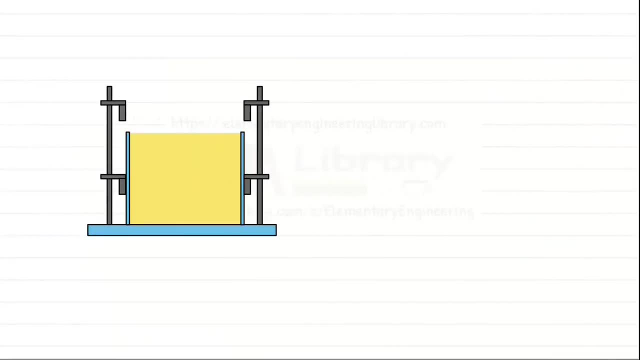 compacted soil in kilo Newton and V is volume of the mould in meter cube. It can also be in ml. We take a representative samples from the bottom, middle and top of the mould and determine the water content of the compacted soil by any of. 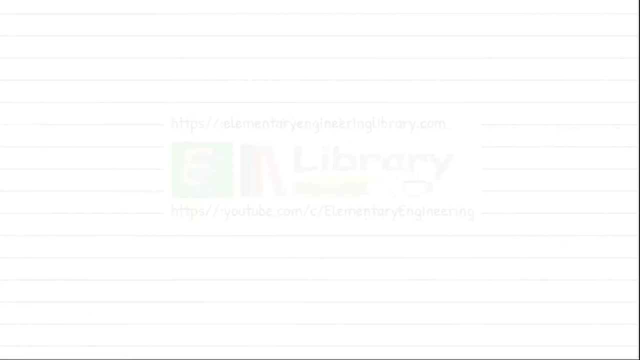 the water determination methods. Once we have the bulk unit weight of compacted soil and its water content, we can calculate its dry unit weight by a known relationship. The soil is removed from the mould and is broken with hands not like this. a little gently, We add more water to the soil so as to increase the 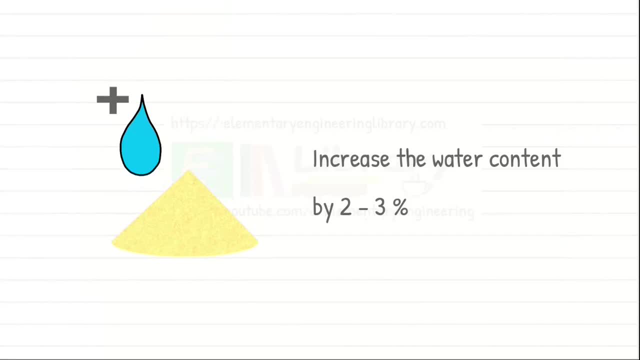 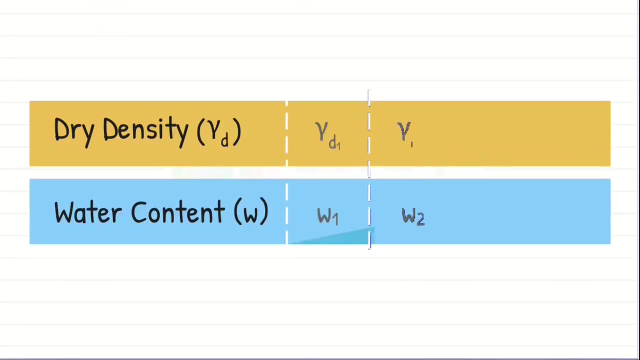 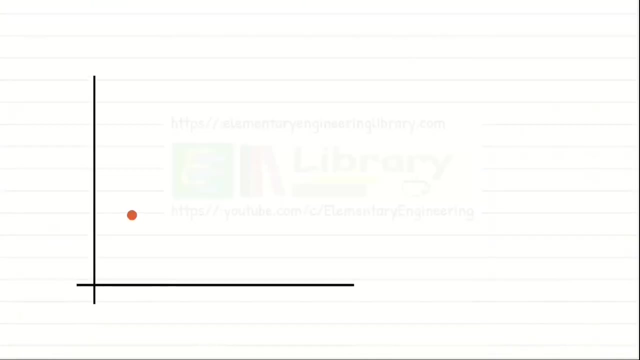 water content by 20%. The soil is mixed and allowed to mature. The whole procedure is repeated and the dry unit weight and the water content are determined. We keep on increasing the water content and determine their respective dry unit weights. We plot these obtained values of dry densities. 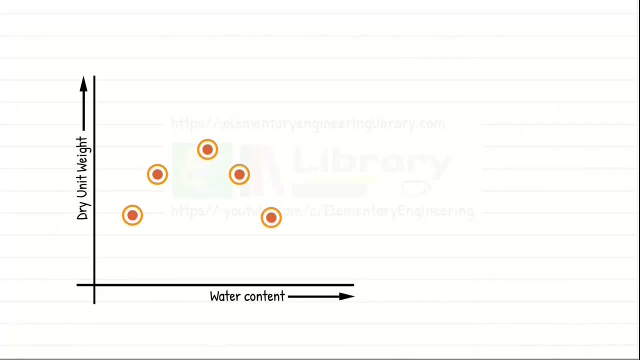 against their respective water contents, and when we join these points together we obtain a curve which is called the compaction curve. Each plotted point on this curve is one compaction test. In the curve we can see that with the increase in water content the dry unit weight of soil initially increases till a maximum value of 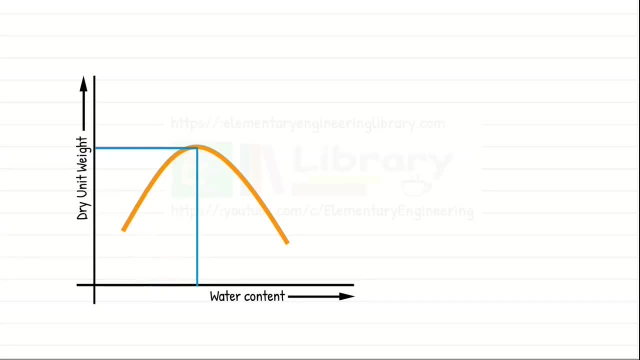 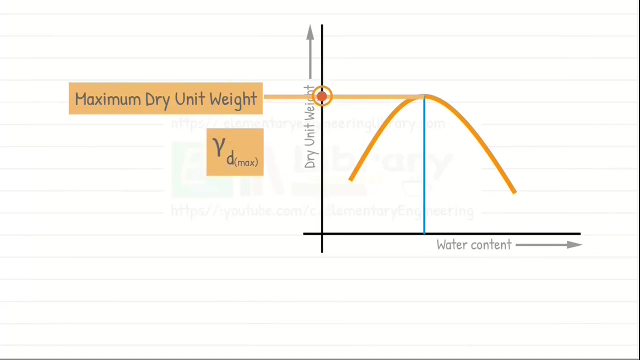 dry unit weight is attained, And if we keep on increasing the water content, the dry unit weight decreases. The maximum value of dry unit weight that a soil achieves is called maximum dry unit weight and is usually denoted as gamma dmax. It is also called maximum dry. 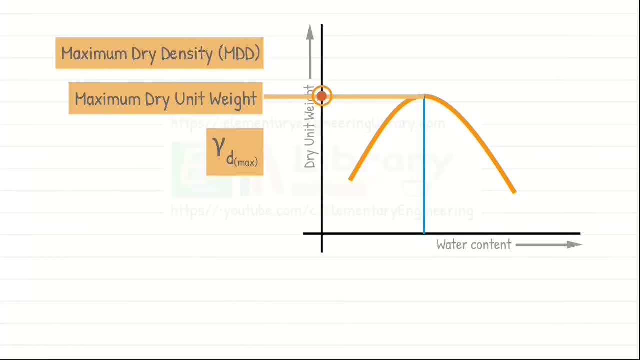 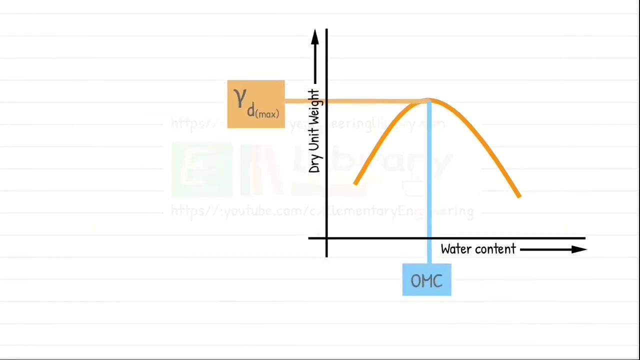 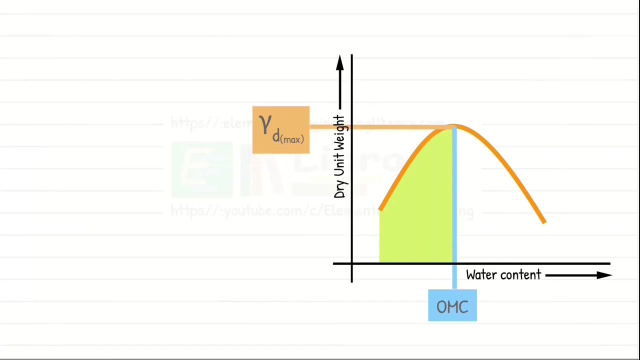 density of soil, Though it is not density, But it is common in soil engineering to use these words unit weight and density interchangeably. The water content at which the maximum dry density is achieved is called optimum water content or optimum moisture content. To the left of optimum moisture content, the moisture content in the soil is less than 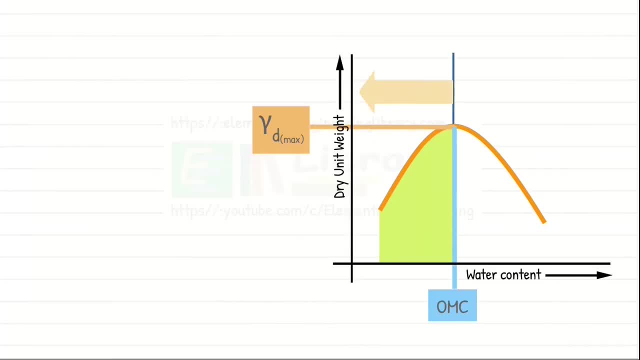 optimum. And this side of curve is known as dry of optimum, Simply because the soil is drier than the ideal moisture content for achieving maximum compaction. In this region the soil is rather stiff and has lot of void spaces, Therefore dry density. 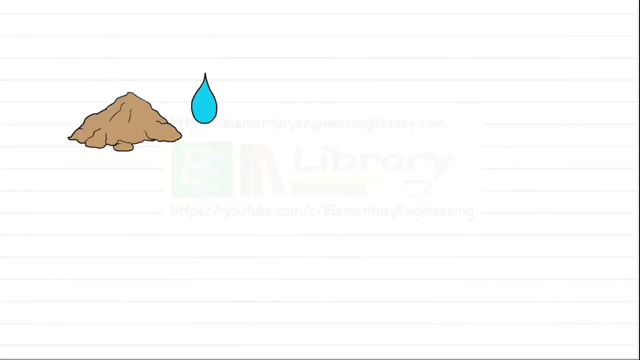 is low. As the water content of the soil is increased, it acts as a softening agent on the soil particles. When load is applied, they slide over each other more easily and move into densely packed positions. Hence, with the increase in water content, the dry unit weight of soil increases. 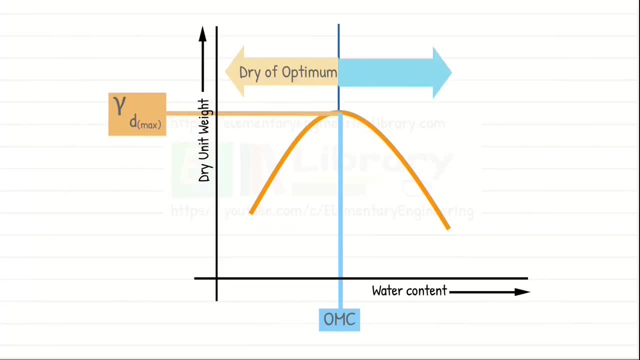 However, to the right of optimum moisture content. water content in the soil is more than the optimum, And this side of the curve is known as wet of optimum. When we keep on adding water content to the soil, the water content in the soil is more. than the optimum, And this side of the curve is known as wet of optimum. When we keep on adding water content to the soil, the water content in the soil is more than the optimum. However, to the right of optimum moisture content, the water content in the soil is more. 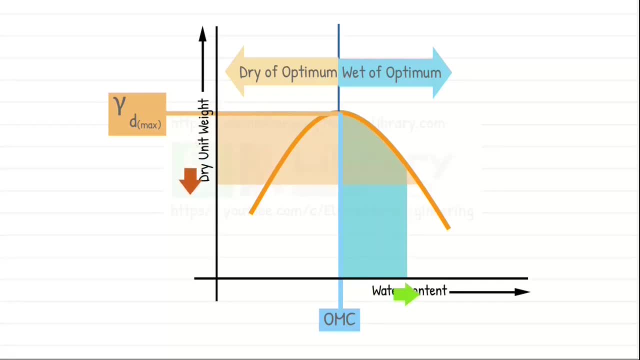 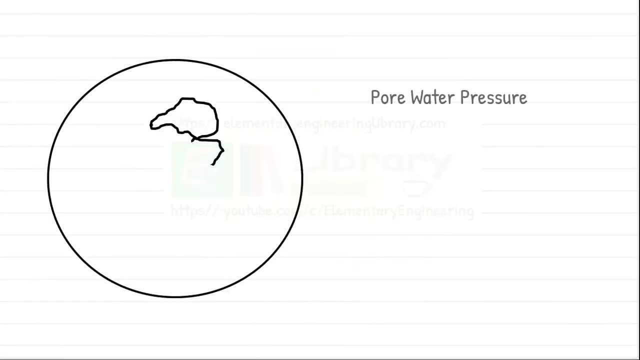 than the optimum. Even after optimum moisture content, the added water results in a reduction in dry unit weight because the pore water pressure, the pressure of water in between each soil particles, will be pushing the soil particles apart, decreasing the friction between them. 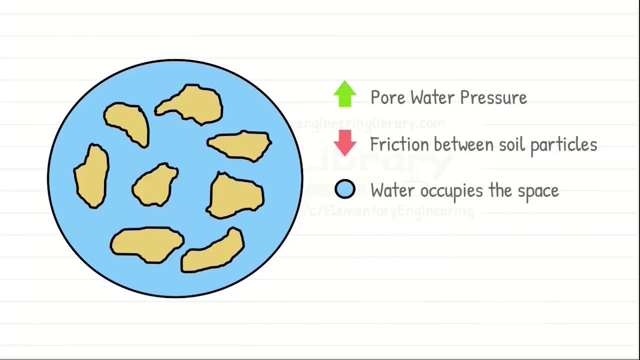 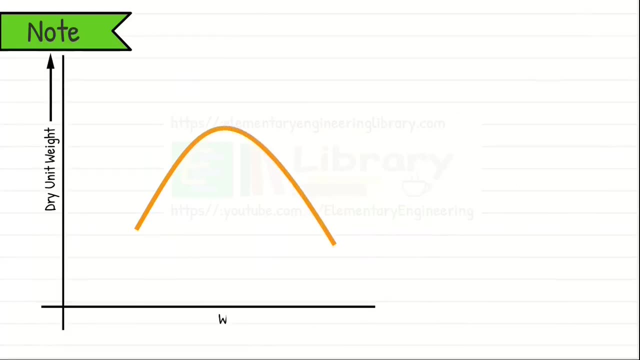 Also, the extra water occupies the space that might have been occupied by the soil particles. Hence, again, dry density of soil becomes low. We should note that this curve is unique for a given soil type, method of compaction and compactive effort. It means if we keep the soil and method of compaction unchanged, but 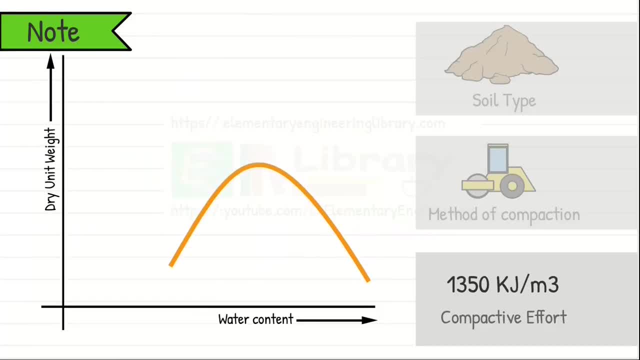 the compactive efforts are increased or decreased, the compaction curve will change. Also, if we keep the compactive effort unchanged but change the soil, the curve will also change. Hence, any particular compaction curve is unique for a particular soil method of compaction. 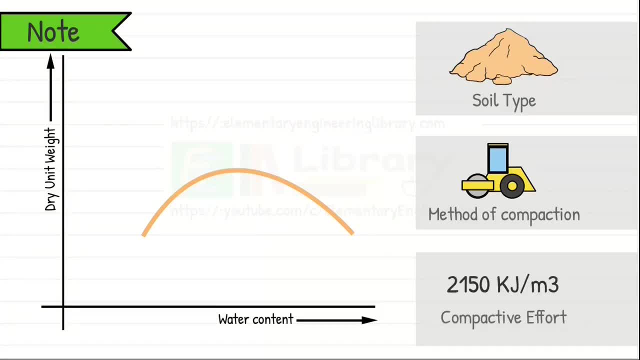 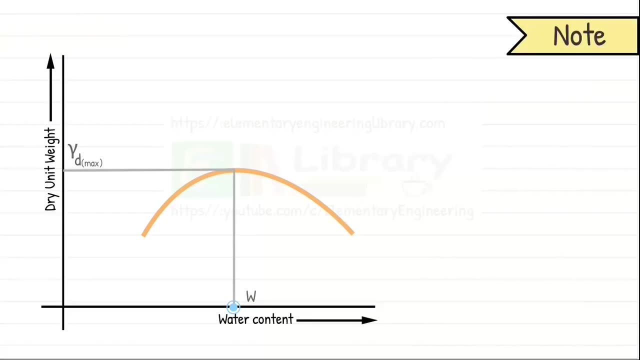 and compactive effort. In the curve we can see that at this water content, soil has achieved maximum water content. Soil has achieved maximum water content. Soil has achieved maximum unit weight or maximum dry density. However, it is important to note that even at this water content, some voids remain within. 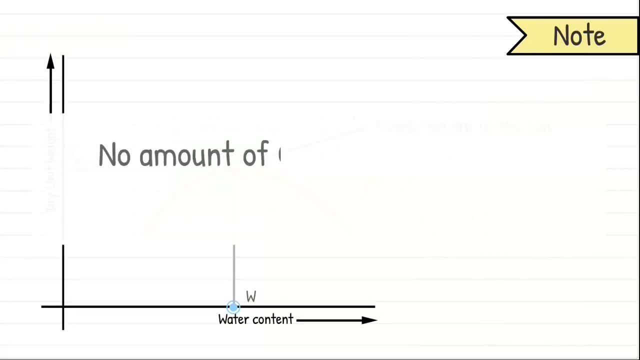 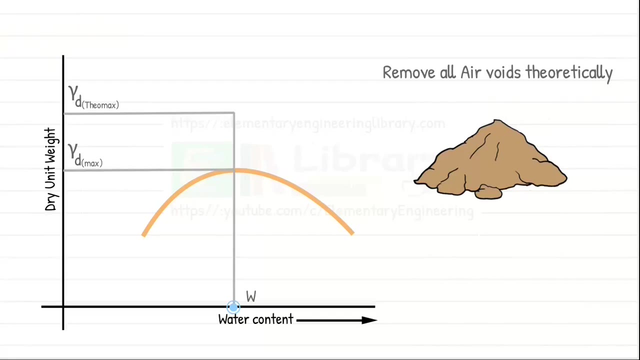 the soil. In fact, no amount of compaction actually removes all the voids from the soil. But if we remove all the air voids from the soil, theoretically the theoretical maximum value of dry unit weight will decrease. But the theoretical maximum value of dry unit weight is only about aatura height, which 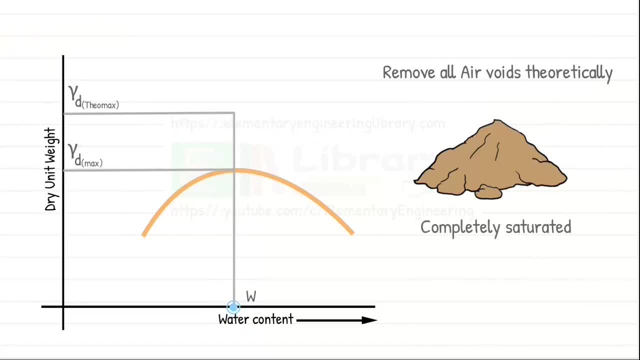 is the maximum idea of the theoretical ambient density impact ratio and flow estimate. Soil is completely saturated and the degree of saturation area is 100%. The parametric티 at this stage is absolutely achieveable. At this time the soil is completely saturated. 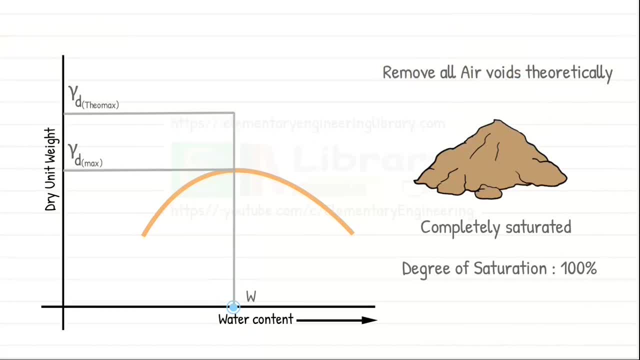 The pista owner also gave a pressüong statement to raise the dist corners and activate the gap of matriculation. Soilleb Within is a Eco-D incent soil. The max humidity is 80 Atchlo water which takes 90 minutes to cool down. atLost air voids. 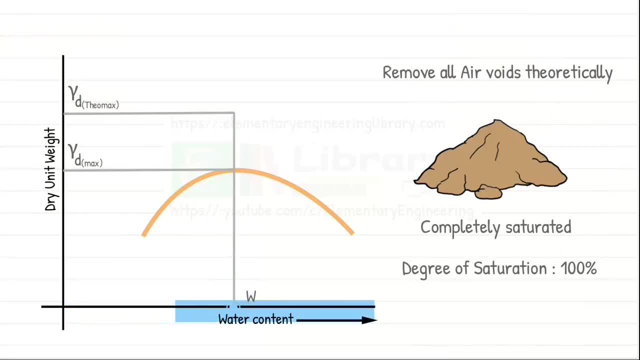 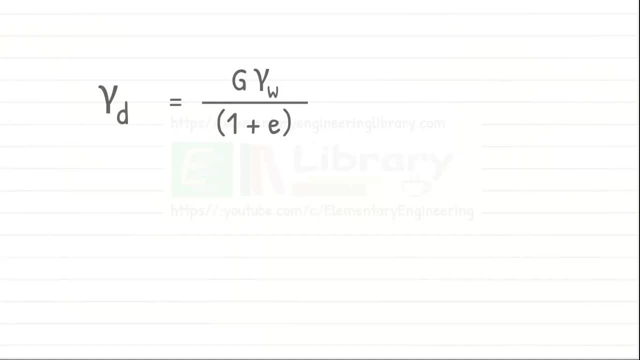 dry unit weight at this or any other water content. we begin with expressing the dry unit weight as a function of void ratio. This is a pre-established equation, derivation of which can be found in our earlier video. link can be found in description. 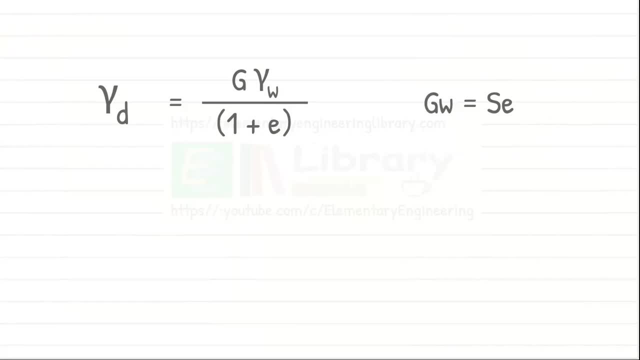 We are also aware of this relationship and the derivation of the same can also be found in that video. From this equation, we can write it to find void ratio, like this, And by substituting it in this equation, gamma d can be written as this: 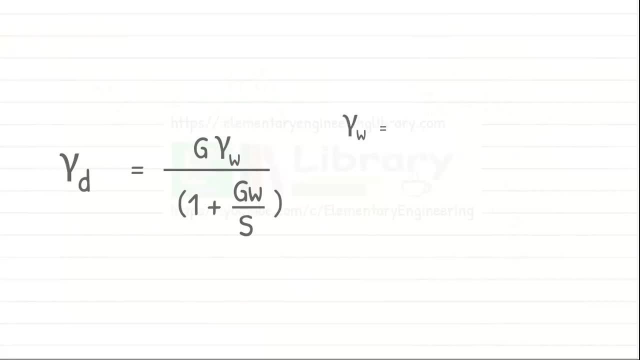 In this equation gamma, w is known as it is unit weight of water, s is degree of saturation and is 100% for calculating maximum value of dry unit weight. Hence we can calculate theoretical max dry unit weight of soil for any value of water content if value of g is known, which 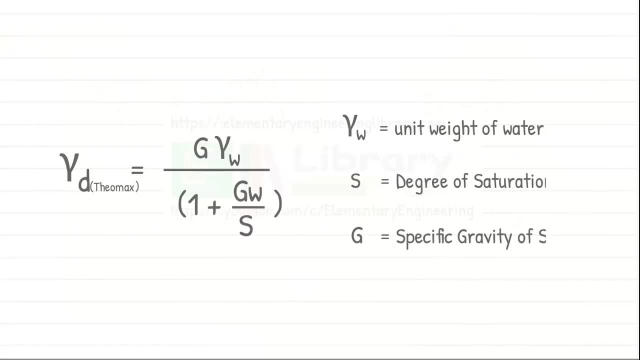 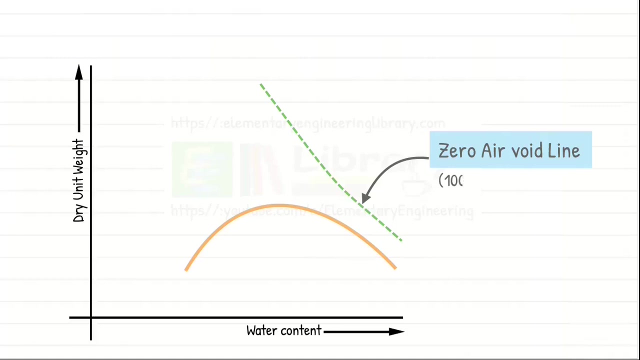 is specific gravity of solids. The line indicating the theoretical max dry unit weight can be plotted along with the compaction curve. It is known as zero air void line or 100% saturation line. We must keep in mind That this curve or line representing 100% saturation is a theoretical limit and is never 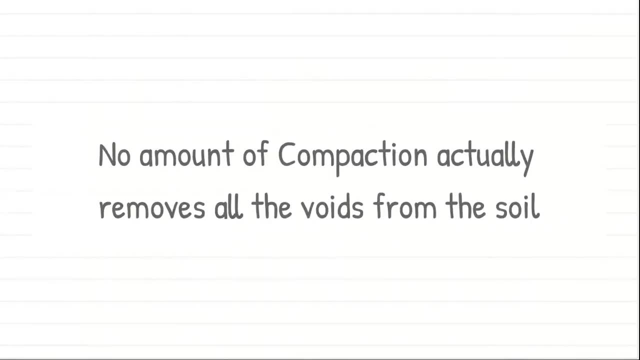 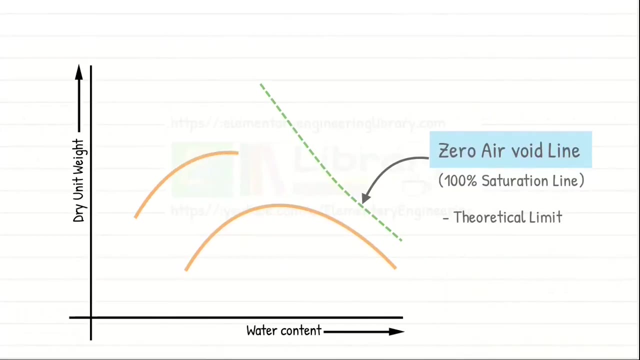 reached in practice, as we have already stated earlier, that it is not possible to remove all the air voids from the soil. One more important thing: When the compaction efforts on soil is increased and a compaction curve is obtained, we observe that the curve has shifted a little upwards and to the left. 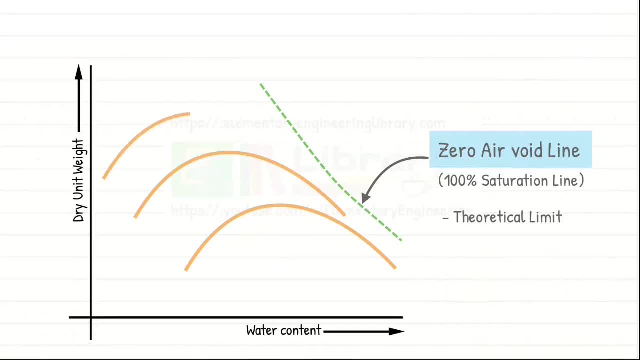 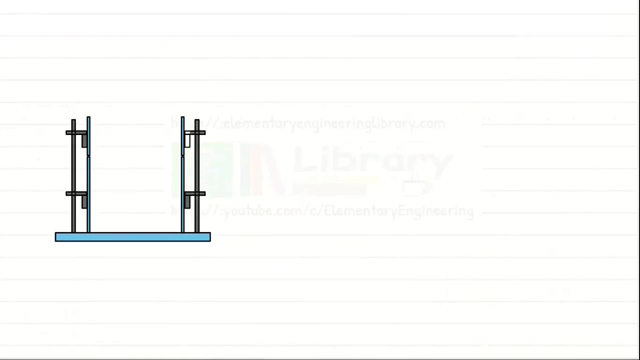 For different compactive efforts we notice a similar shifting of the curve. And when we join the peaks of these compaction curves, a line of optimus is obtained. Well, that is standard proctor test and analysis of its results. The purpose of this test. 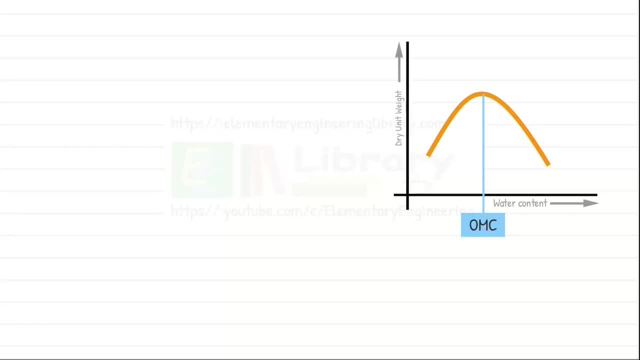 Is to find out the optimum moisture content at which soil achieves its maximum dry density or maximum unit weight. Then, in the field, our goal is to achieve soil density as close as possible to the maximum dry density obtained via laboratory test In India. the Indian standards recommends a test for compaction. 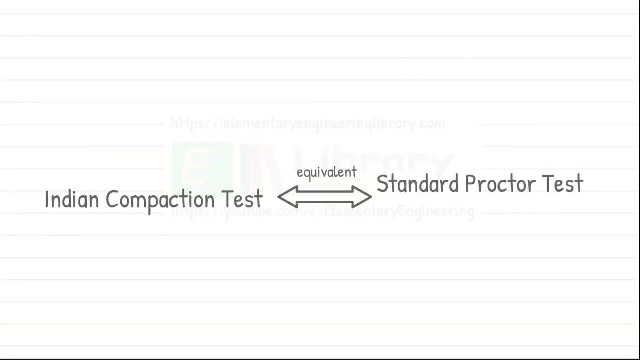 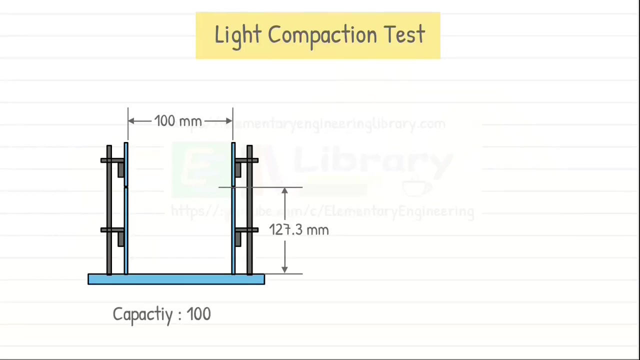 That is equivalent to the test for compaction. It is called the standard proctor test and is called light compaction test. There are only minor modifications to the test. It recommends the mould of 100 mm diameter, 127.3 mm height and 1000 ml capacity. 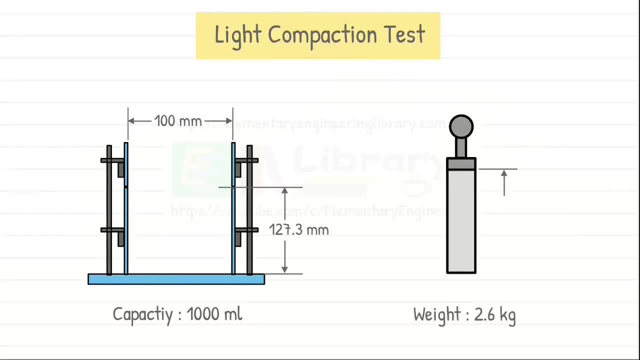 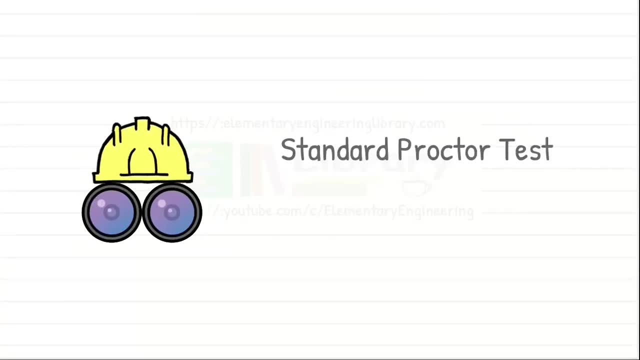 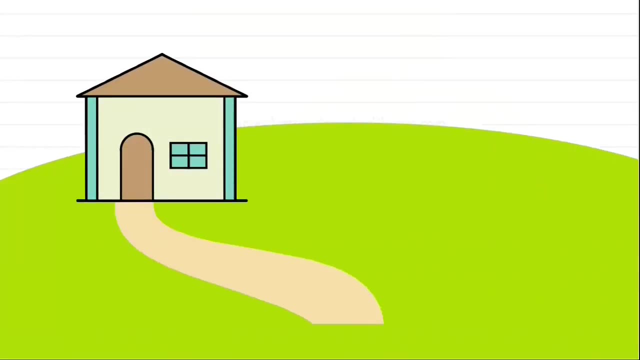 Also, the rammer is of 2.6 kg and the free drop is 310 mm. It was observed that the standard proctor test Is better suited for smaller projects, Like construction of small building, garden, pathway, small retaining wall, etc. 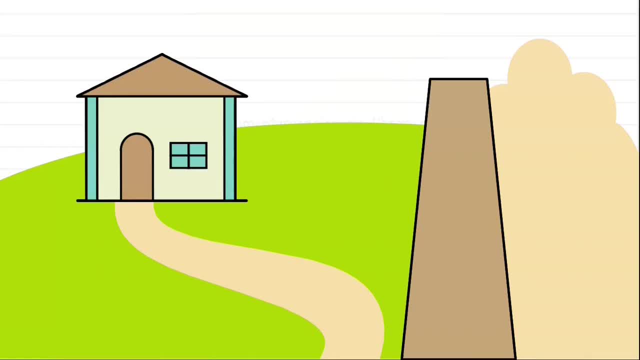 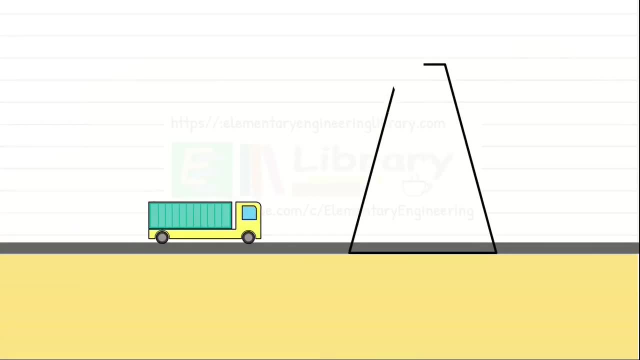 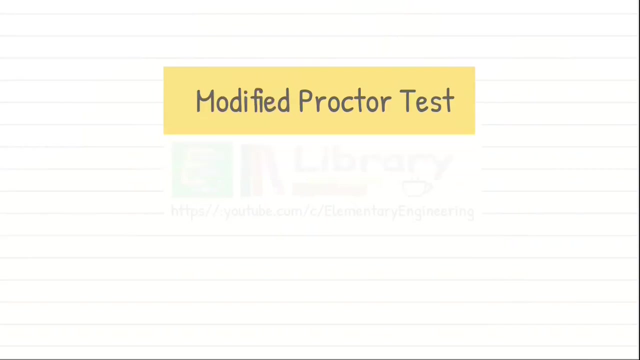 Where loads on soil are not substantial, But for projects that need heavy compaction of soil, Such as construction of highways, dams, etc. The standard proctor test does not represent the true compaction characteristics For such conditions. The standard proctor test has been updated into the modified proctor test. 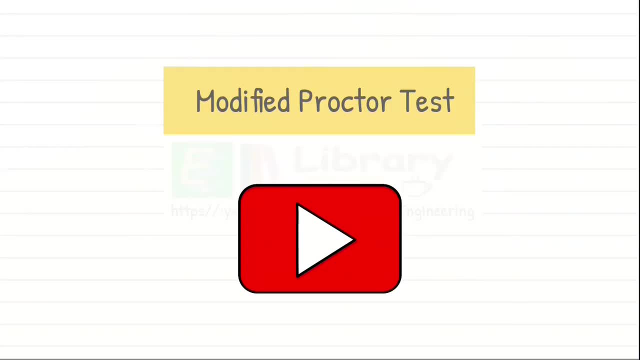 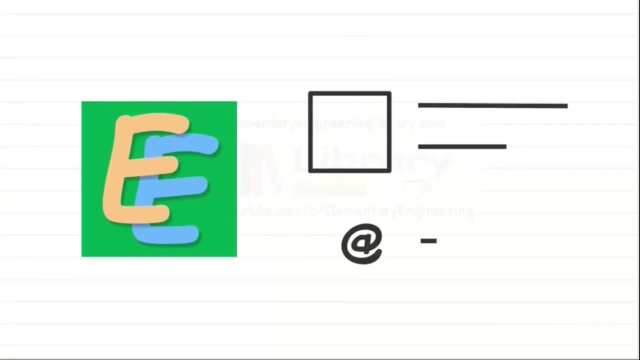 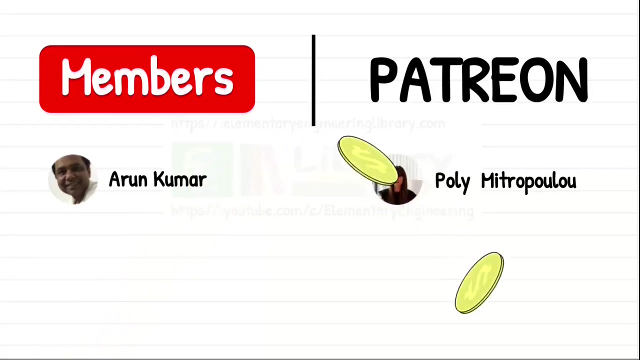 And that we will discuss in the next video. Elementary engineering receives lots of love via beautiful comments and lovely emails. Thank you everyone for showing your love to this channel. Also, thank you very much, members and patrons of elementary engineering, for supporting this channel monetarily. 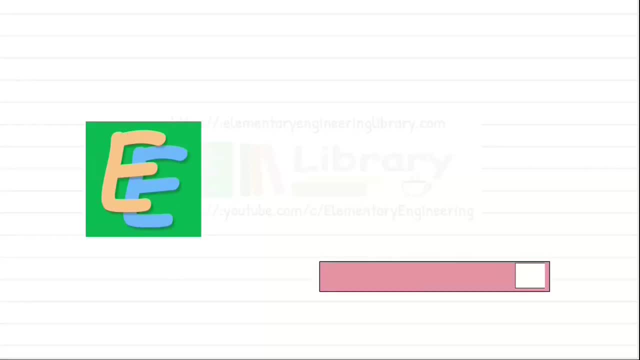 If you think elementary engineering has given you knowledge that worth something to you, Consider supporting this channel by becoming the member of this channel here on youtube, or you can also consider becoming a patron on patreon. Elementary diaries are back in the professor's store.